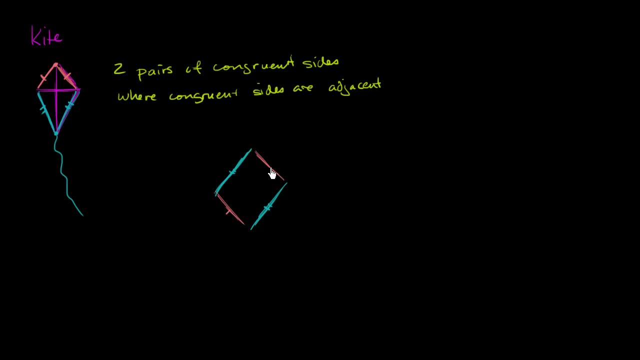 that is congruent to this side. This would be a situation where you have two pairs of congruent sides but they're not adjacent. They don't have any common endpoints with each other. Each side in the congruent side pair. they are opposite to each other. 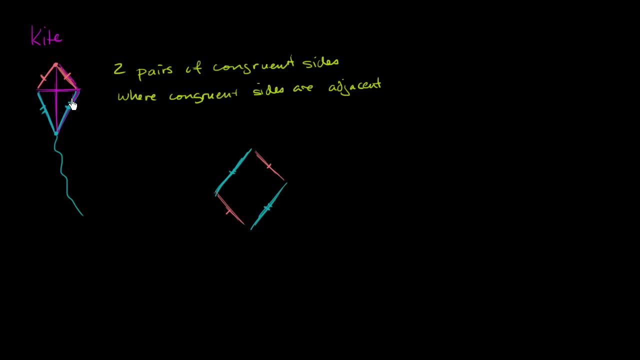 So here once again, we get a quadrilateral. We still get four sides. A kite is a quadrilateral, This is a quadrilateral, But this isn't a kite. This right over here is a parallelogram, And we've seen that multiple times before. 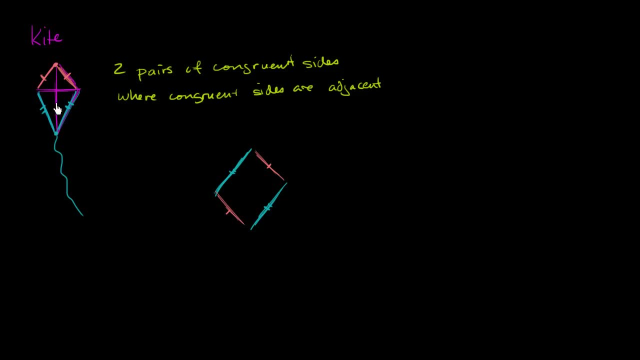 But kites can also be constructed in other interesting ways. You might see that what looks right here, that these two diagonals of this kite are perpendicular And that indeed- and I'm not going to prove it here- is a property of a kite. 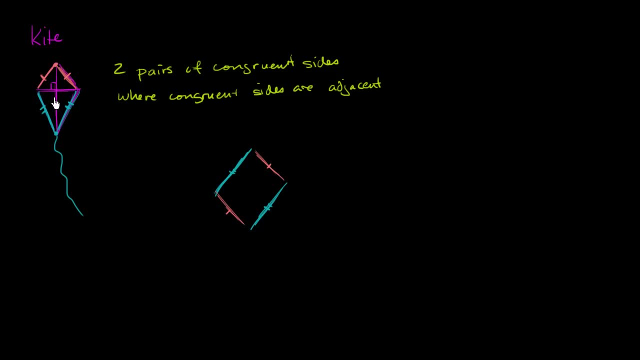 This right over here. these two lines, these two diagonals, intersect at a 90 degree angle. The other thing we know about kites is that one of these lines is bisecting the other of the two, So you could actually construct a kite that way. 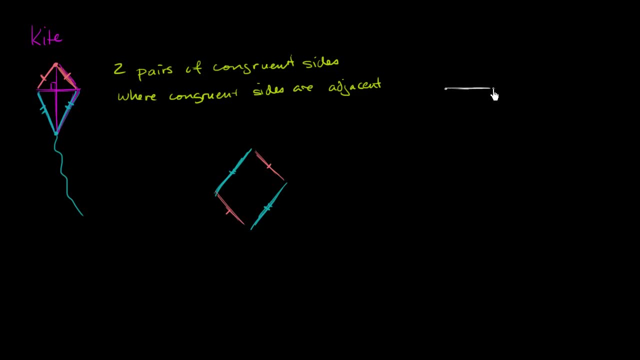 You could start with a line and then you could construct a perpendicular bisector of that line, another segment that bisects it at a 90 degree angle. So here, there you go. So that bisects it. So that means that this segment is equal to this segment. 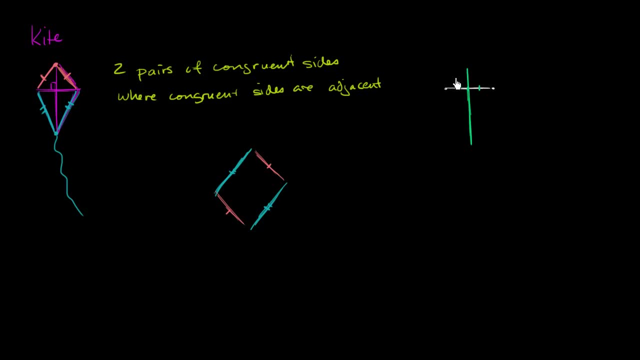 We split it in two And then, if you connect the endpoints of the segments, you should get a kite, And you will indeed get a kite. So it would look something like this And, once again, this segment is congruent to this adjacent segment. 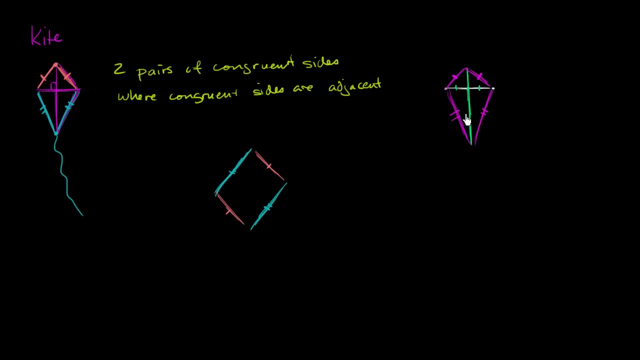 And this segment is congruent to this adjacent segment. But what would happen if these two diagonals are both perpendicular bisectors of each other? So what would happen in this scenario Where let me draw one segment And then I'm going to make? 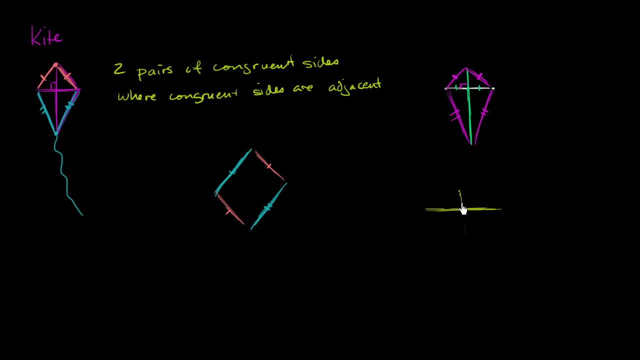 another segment, But they're going to be perpendicular bisectors of each other, So let's do that. So now they're both perpendicular bisectors of each other, So this segment is equal to this segment And this segment is equal to this segment.